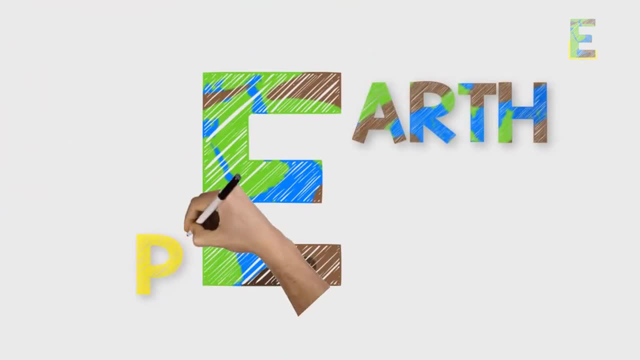 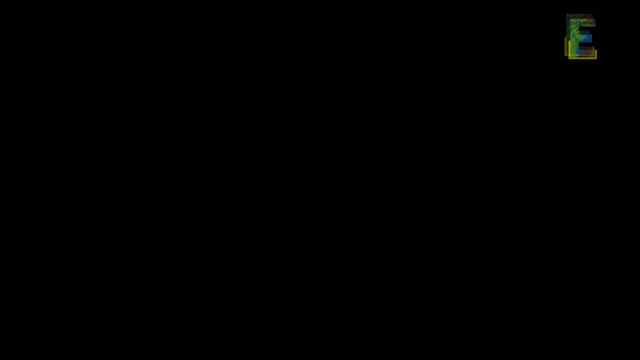 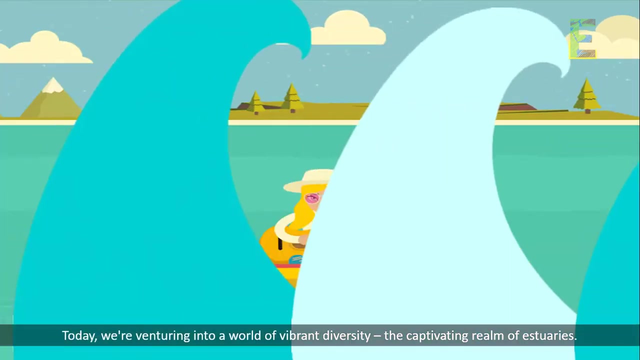 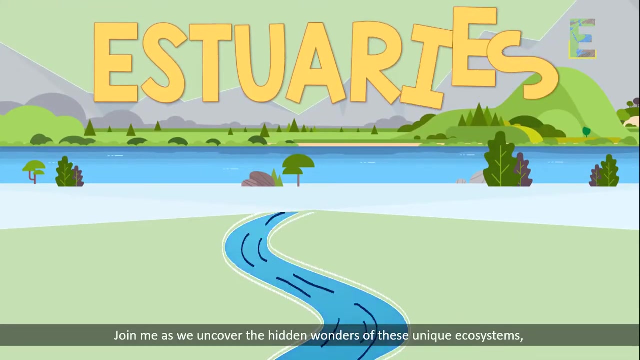 Greetings nature enthusiasts. Welcome back to our channel. Today we're venturing into a world of vibrant diversity: the captivating realm of estuaries. Join me as we uncover the hidden wonders of these unique ecosystems, where the dance of saltwater and freshwater creates a 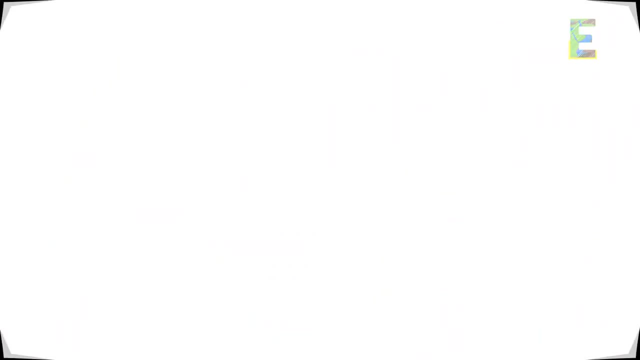 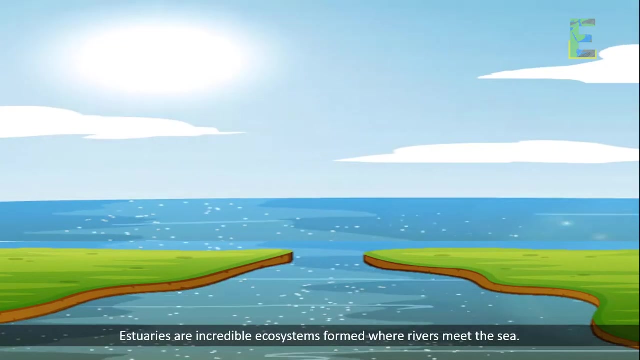 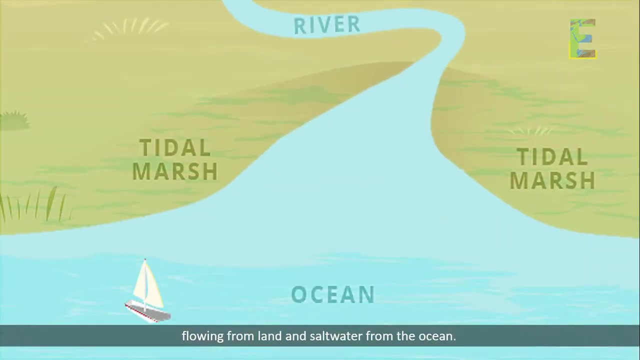 symphony of life. Let's dive in Defining estuaries. Estuaries are incredible ecosystems formed where rivers meet the sea. These transitional zones are a result of the interplay between freshwater flowing from land and saltwater from the ocean. Estuaries come in various shapes. 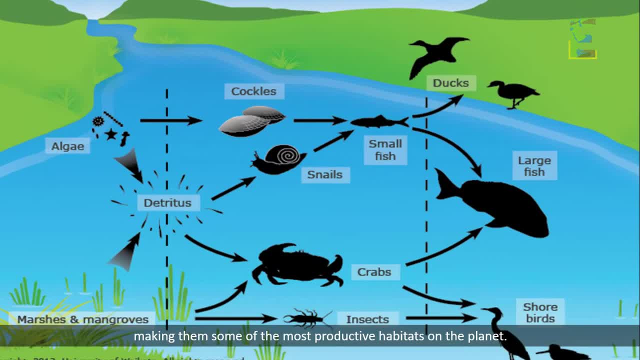 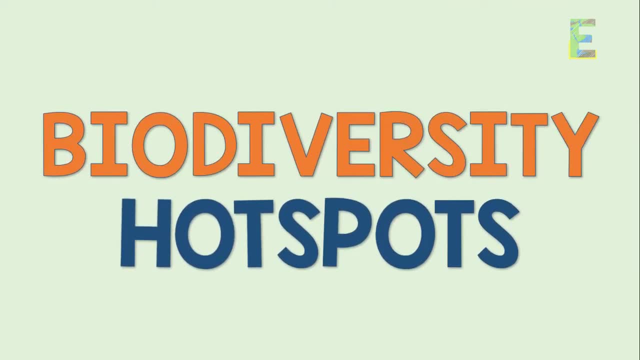 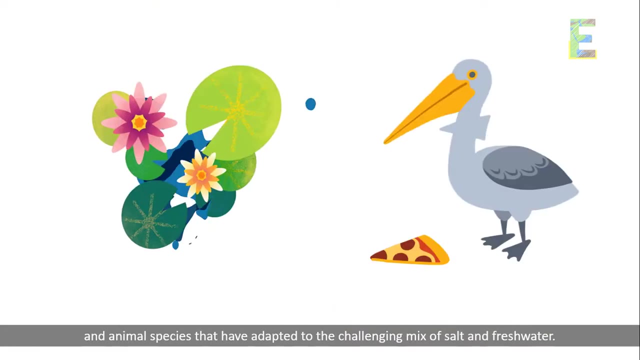 and sizes, and they're teeming with life, making them some of the most productive habitats on the planet. Biodiversity hotspots- Estuaries are true hotspots for biodiversity, hosting a plethora of plant and animal species that have adapted to the challenging mix of salt and freshwater Mangroves. 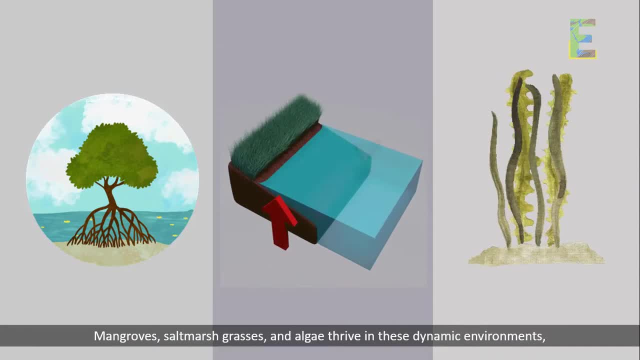 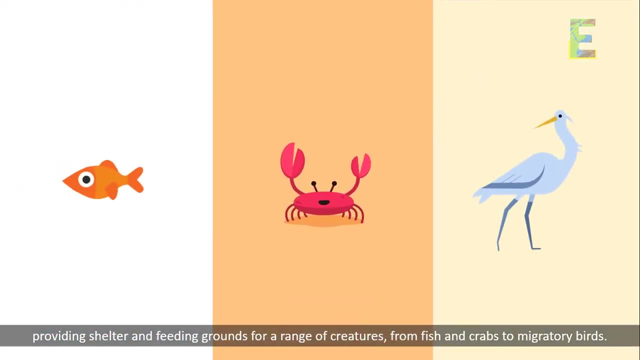 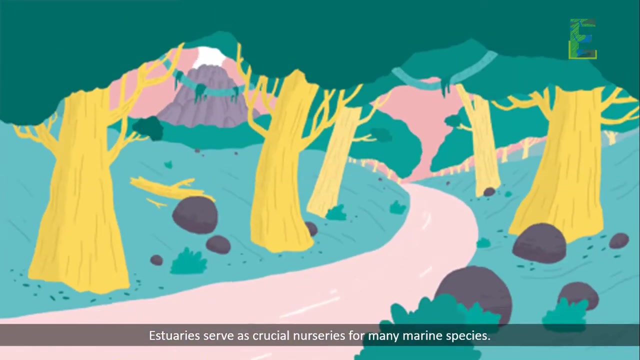 saltmarsh, grasses and algae thrive in these dynamic environments, providing shelter and feeding grounds for a range of creatures from fish and crabs to migratory birds. Nurturing ground animals, Estuaries serve as crucial nurseries for many marine species. The mix of nutrient-rich 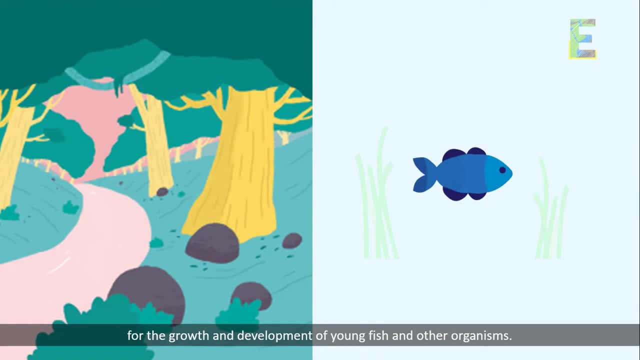 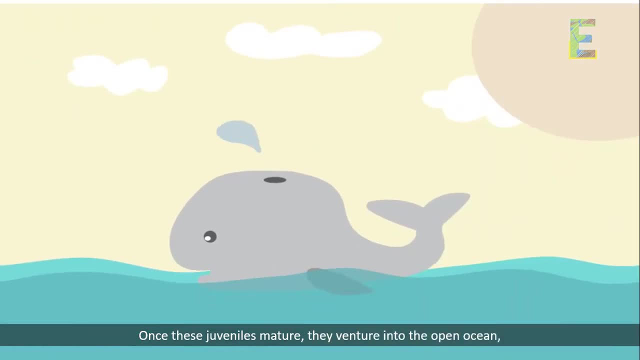 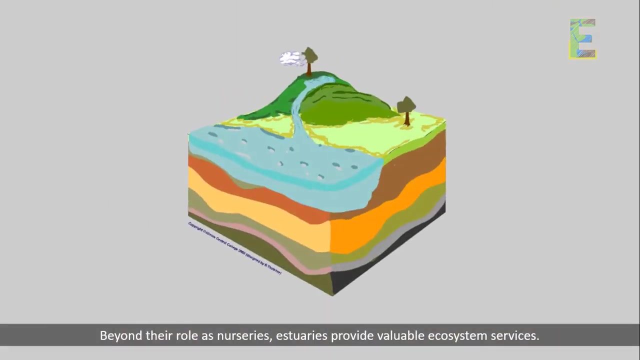 waters and protective habitats makes these areas ideal for the growth and development of young fish and other organisms. Once these juveniles mature, they venture into the open ocean, contributing to the larger marine ecosystem, filtering and buffering beyond their role as nurseries. 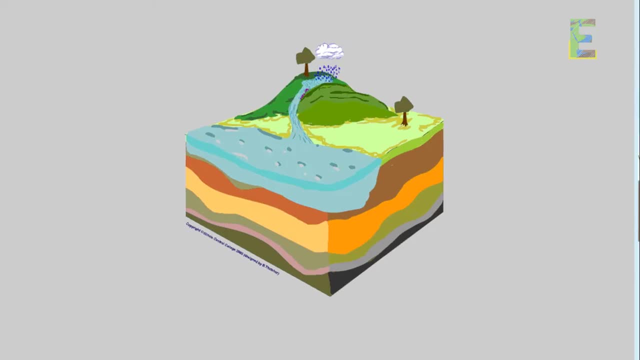 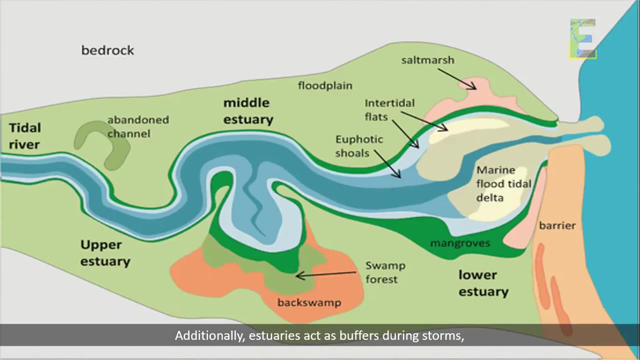 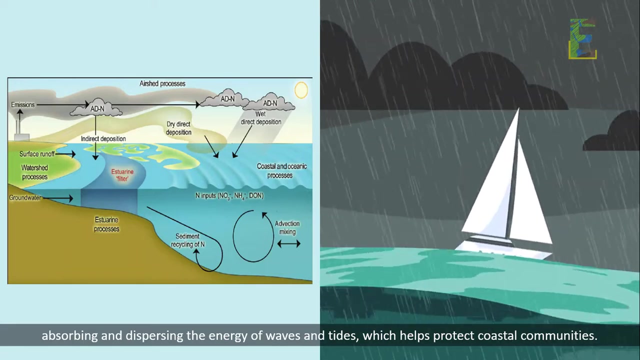 Estuaries provide valuable ecosystem services. They act as natural filters, trapping sediment and pollutants from land before they reach the sea. Additionally, estuaries act as buffers during storms, absorbing and dispersing the energy of waves and tides, which helps protect coastal communities, threats and conservation, While